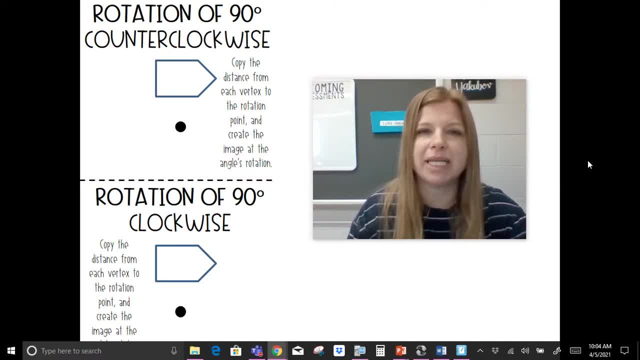 you would still follow the same formatting, but where you see me drawing the angle measure of 90 degrees, you would simply to adjust it to whatever other, whatever measure. you need to do. So if I say to you: rotate a figure Now, in general rotations are always counterclockwise and counterclockwise. 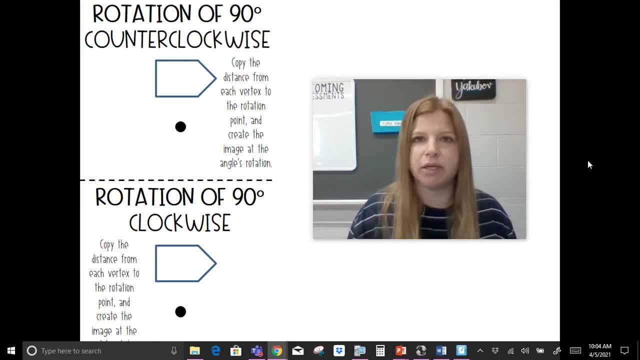 means it goes to the left. So picture you know you're at a steering wheel. you would if you were turning that steering wheel to the left. that would be the counterclockwise motion. Clockwise also is just how a clock goes. Clockwise would be: you know how a clock go- the hands. 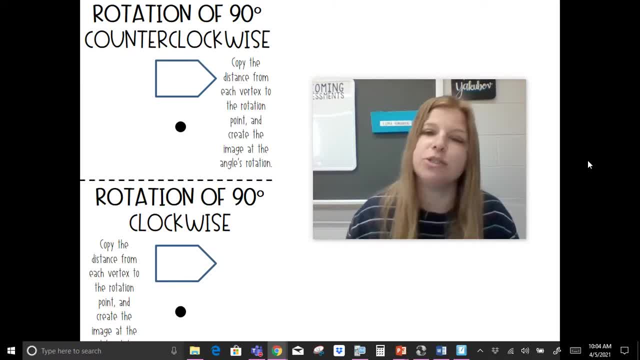 go around the clock. So counterclockwise, of course, is the opposite way to the left. So if I said to you, I wanted you to rotate this figure here, this pentagon, counterclockwise 90 degrees, What we really are doing is we are drawing a segment from that point to each vertex of this pentagon. 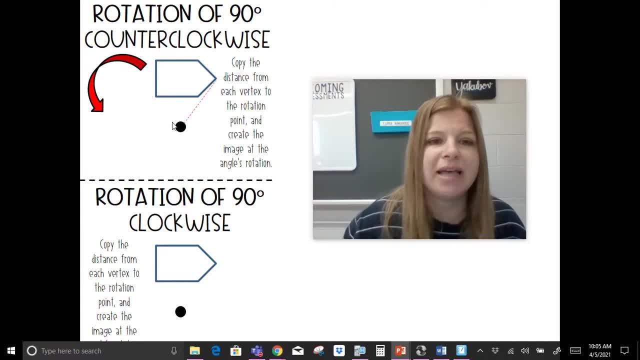 And what we would need to do is we would need to take that length that we are trying to rotate. Okay, so from this point to this point on the vertex- And I'm going to copy that distance at a 90 degree angle going to the left, To the left, It's reversed on my screen. 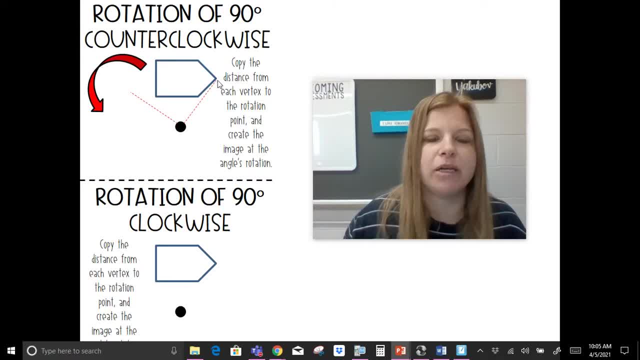 So if I was to do that, from this point going towards the left, copying that same length at a 90 degree angle, this point here would get rotated to this point here. Okay, so I measure the distance from the point to the left And I'm going to copy that distance at a 90 degree angle, going to the left, And I'm going to copy that. 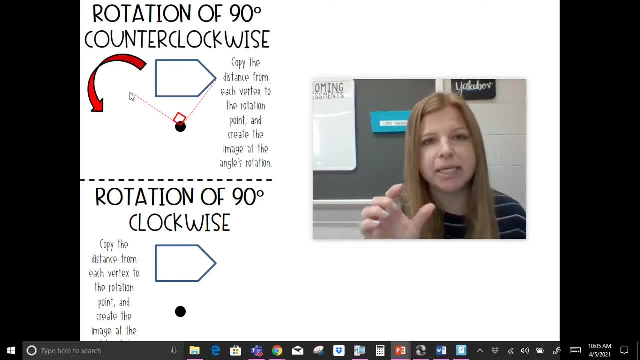 to that vertex. I map out a 90 degree angle and I copy that same segment over 90 degrees going to the left, And then I would do that with the next point. So let's say I've connected the point to this vertex. 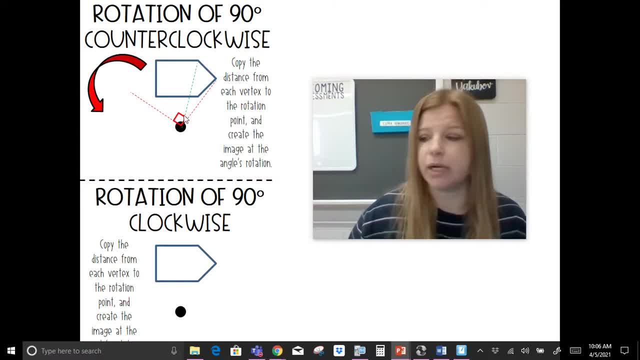 I measure that length. I take my protractor or a corner. You can always take a piece of paper, guys. A post-it works out really, really well because obviously that's 90 degrees. Make a little marking on the post-it. You know how far you went for that segment. Use the corner. 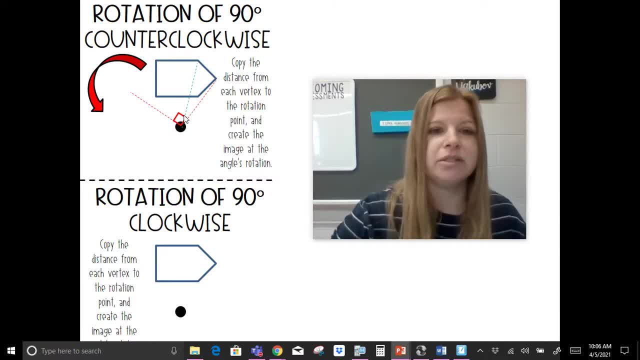 To create your 90 degrees and then copy that segment. So if I took that green length there and I copied it at a 90 degree angle, those two points would be there. Now, of course, I would do the same process with the other three points on this pentagon and I would end up getting my image. 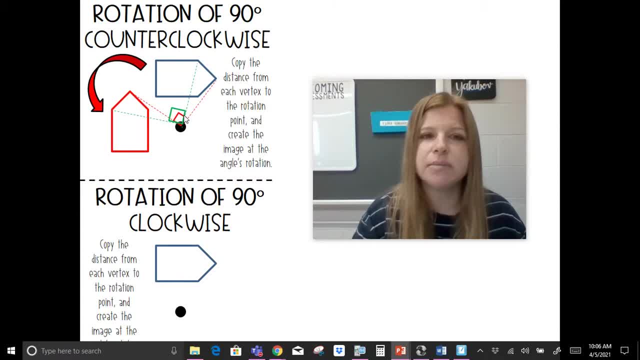 there. So that's what a rotation of 90 degrees looks like And some things to notice. Notice the blue original pre-image looks like it's kind of a pentagon sitting on its side And then, when it got rotated, it's now pointing upwards. So that's not a coincidence. So I'm going to copy that segment. 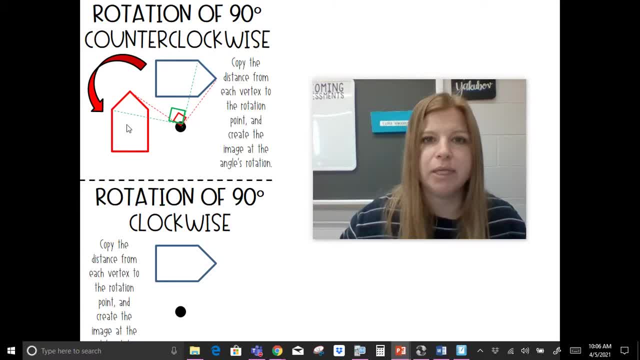 and I'm going to rotate it 90 degrees, So that's not a coincidence. You can also then picture where this figure would be. if I took the red image and now rotated it 90 degrees, It would be down here and it would be pointing to the left. And if I took that figure rotated another 90 degrees then 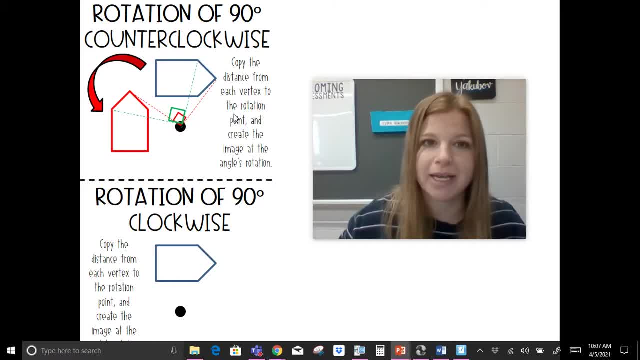 it would be here pointing downwards. And if I rotated it one more time, guess what? four rotations of 90 degrees gives you 360 and you'd be right back where you started. Clockwise just means we're going into, we're going to the right this time. Okay, so just the way. a clock, the hands go around. 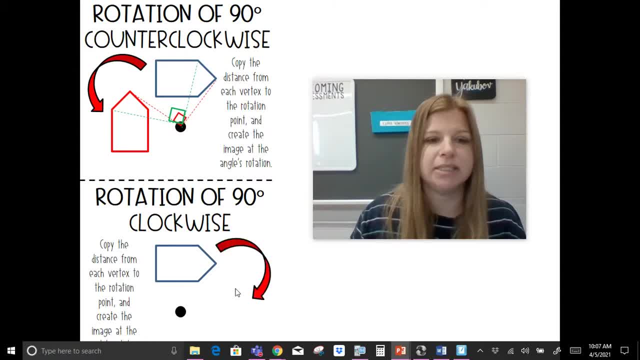 the clock, I would still do the same process. So if I took the red image and now rotated it 90 degrees, I would still copy the distance from each vertex to that point at a 90 degree angle And that would be where my new that would be where the image point would be, And I would do that for each one. 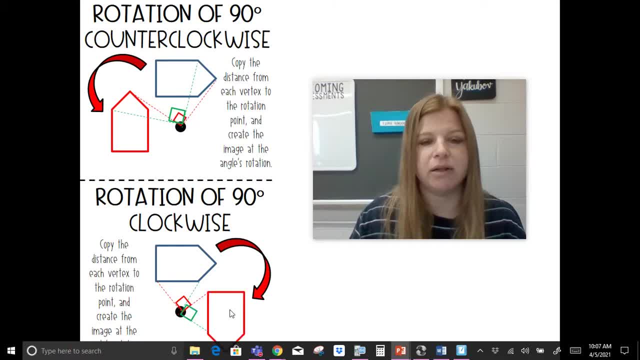 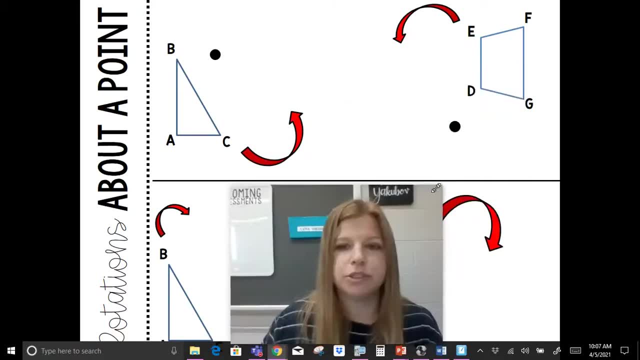 of these vertices at a 90 degree angle, until I've completely copied my figure. Okay, so at the top, I'm going to show you what it looks like to rotate these counterclockwise, which is the natural way of any rotation. You only ever rotate them counterclockwise. You only ever rotate them counterclockwise. 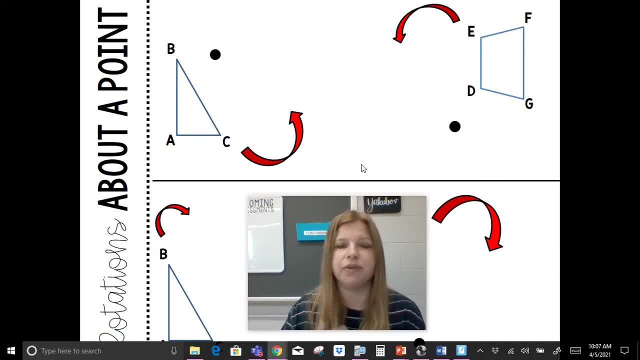 If it just says rotate the figure, then it's always by default counterclockwise. So if I want to take this triangle ABC, rotate it 90 degrees, counterclockwise, I would measure my length from A to the point. Okay, measure this length with a ruler. post-it note. make a little notch on the post-it note. how long? 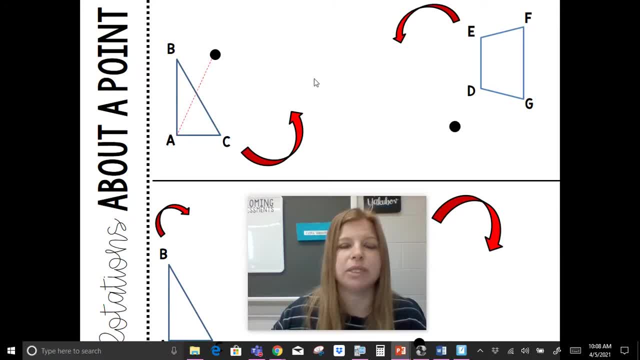 far it is. Make a 90 degree angle going towards the left. So that's how we're turning towards the left. Map out the same distance and then I'm going to rotate it 90 degrees counterclockwise. So if I want to rotate it 90 degrees counterclockwise, I'm gonna measure the distance, and so that's where my A.